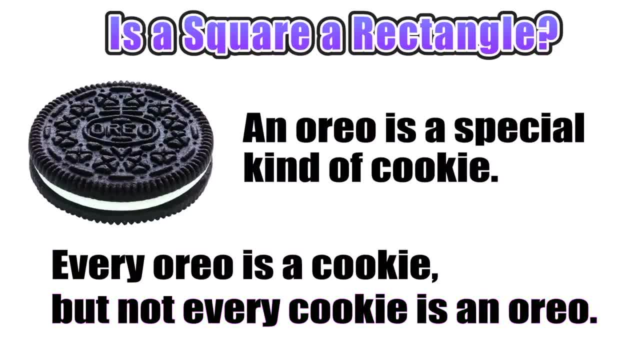 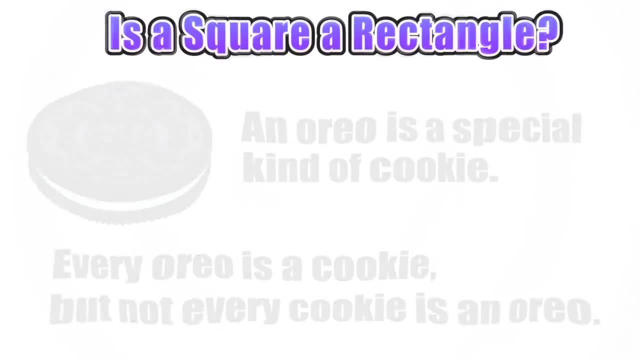 but not. every cookie is an Oreo. So, believe it or not, we just engaged in mathematical reasoning And now we're going to take that same kind of thinking and apply it to our original question: is a square, a rectangle? So let's go ahead and start off with the definition of a cookie. 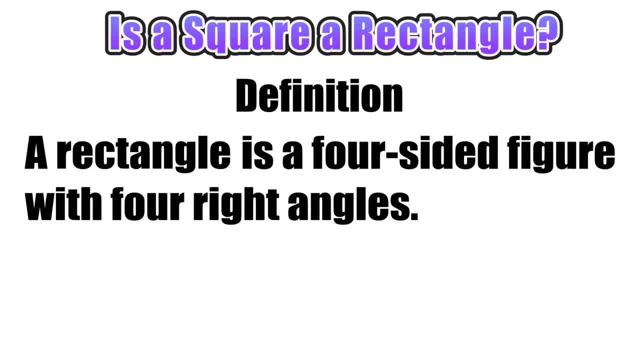 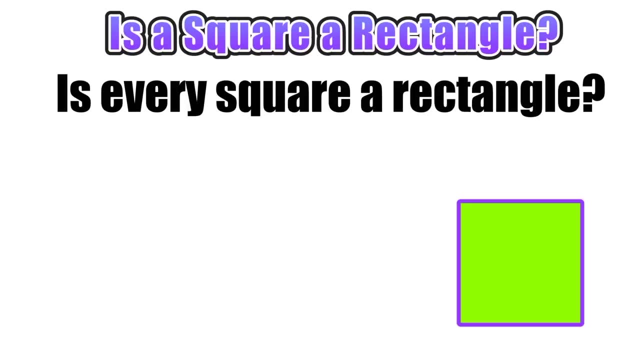 So let's take a look at the definition of a rectangle, which is a four-sided figure with four right angles, And again we want to see if a square will satisfy this definition and allow us to answer the question: is every square a rectangle? Now, we are all familiar with squares. 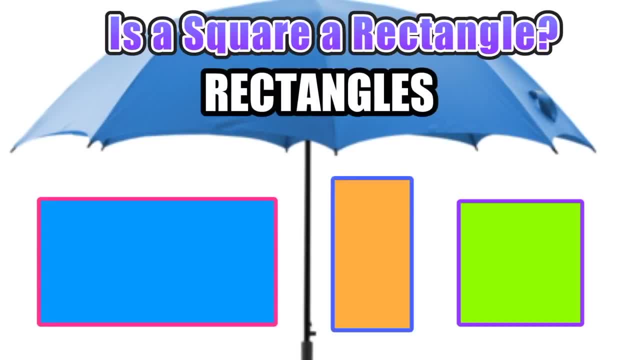 and rectangles, and we can easily draw four-sided figures with four right angles that would be considered rectangles and satisfy our definition. I'm sure that you can also draw a square with four right angles, and you can also identify four-sided figures that are not rectangles, namely a. 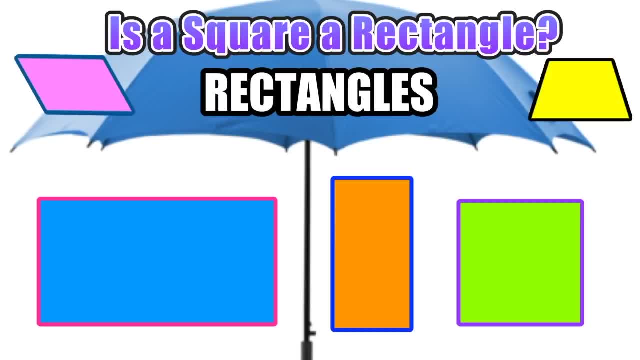 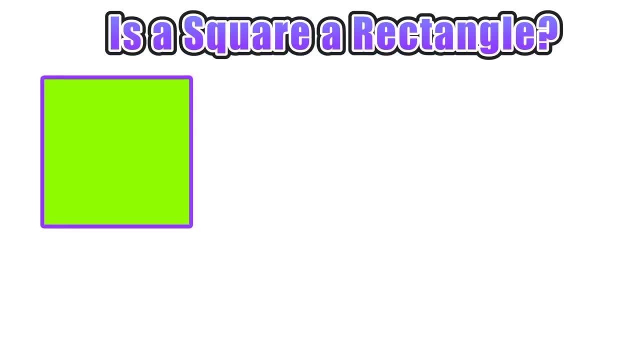 parallelogram or a trapezoid, because they do not have four right angles. Now remember, since the square satisfied the definition of a rectangle, we can say that a square is a special kind of rectangle, And what makes it special is not the fact that it has four right angles, but the fact 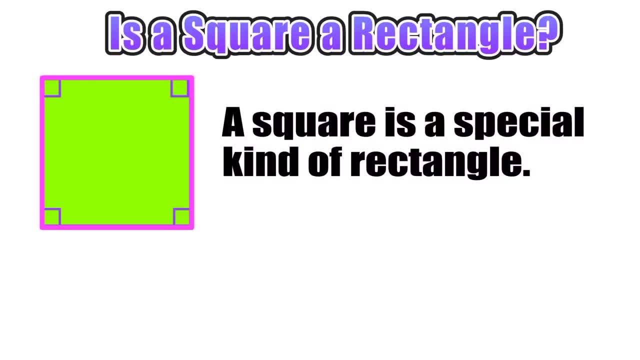 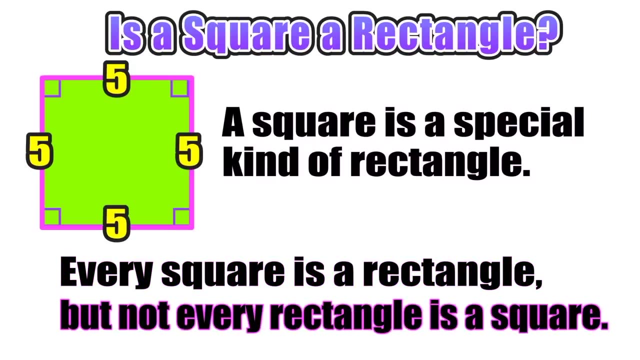 that it has four equal sides. So all the sides are equal. So we can say that a square is a special kind of rectangle. So if you knew that one side of a square was five, you would know that all the sides must be five. So we can conclude that every square is a rectangle, but not every rectangle is. 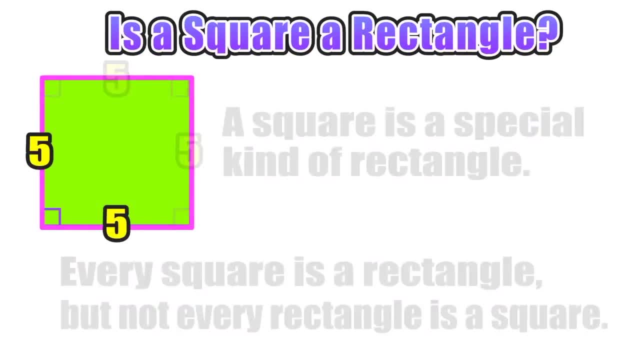 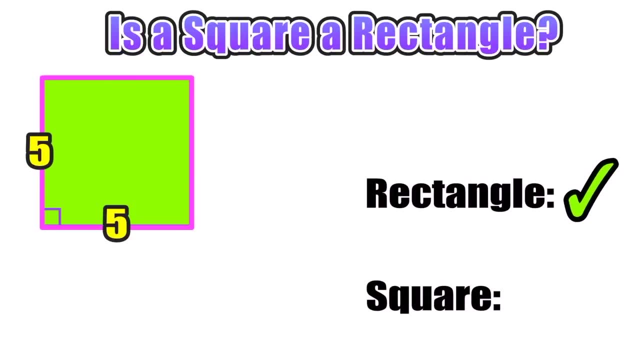 a square. So when you're asking yourself this question and you have a figure like the one shown, if it has four right angles and four sides, then you can conclude that the figure is a rectangle, And if those four sides are all the same length, then you can conclude that the figure is. 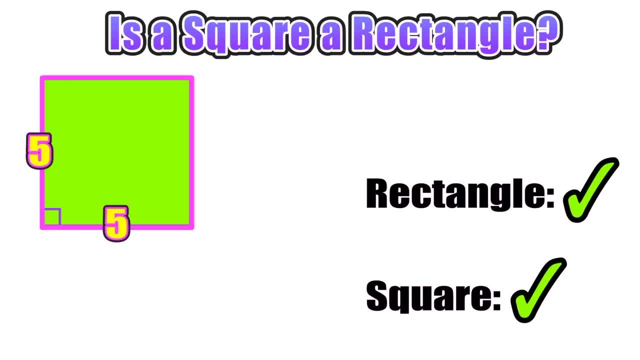 a square. Remember that a square is a special kind of a rectangle, But also remember that not every rectangle is a square. If we extend our figure and double the length from five to ten, it still represents a rectangle. but this is not a square, again, because the side lengths are not the same.